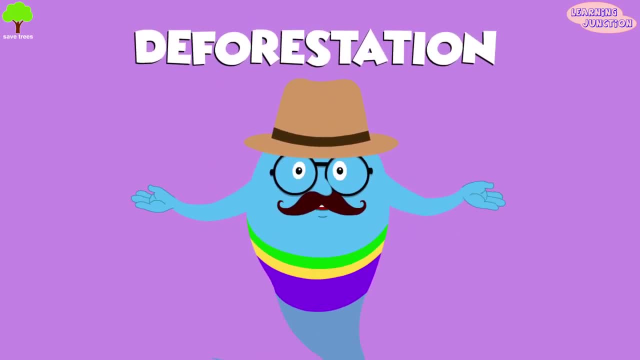 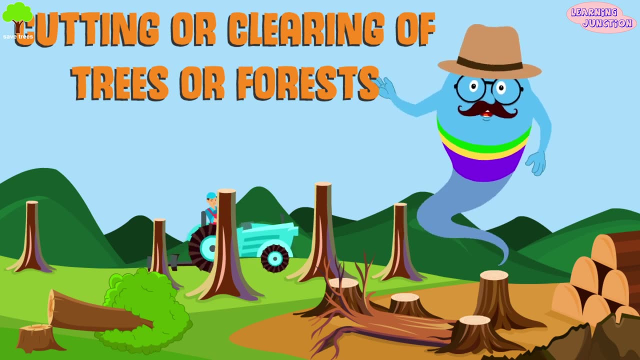 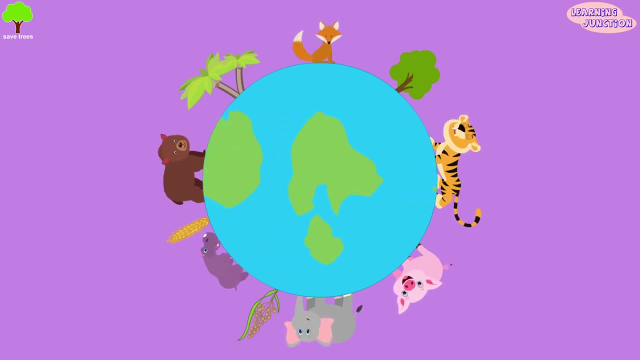 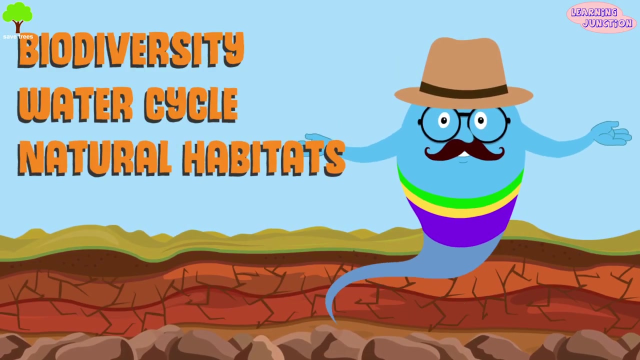 Hello friends, today we'll learn about deforestation. Deforestation means cutting or clearing of trees or forests over a large area for the facilitation of human activities. It is a serious environmental concern, since it can result in the loss of biodiversity, disturbances in the water cycle, damage to natural. 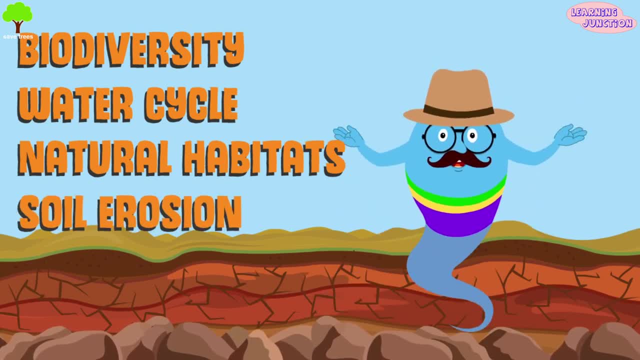 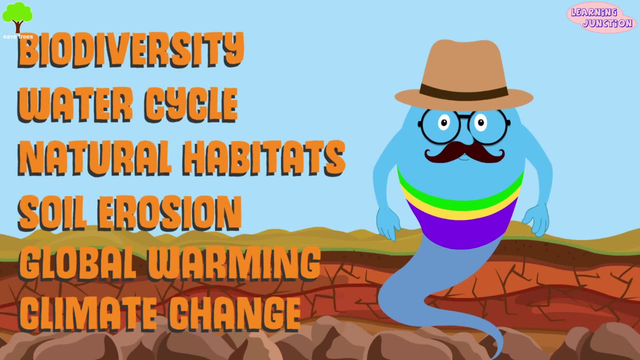 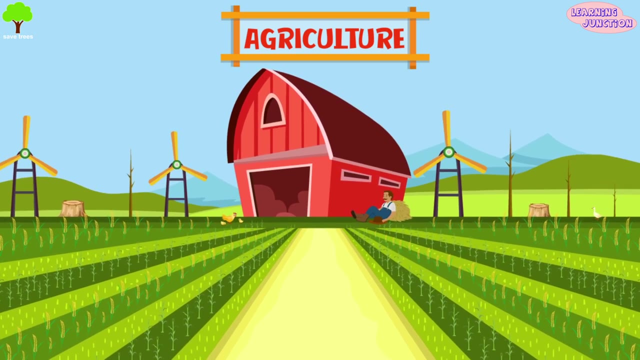 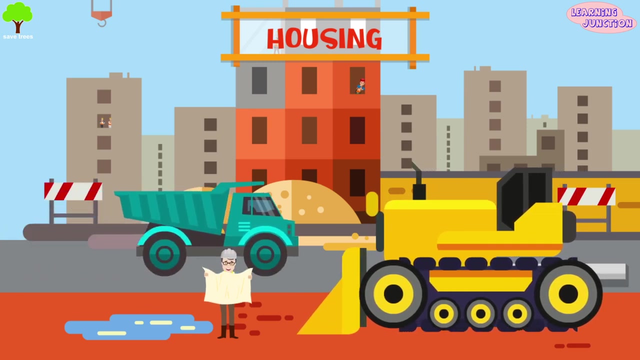 habitats and soil erosion. Deforestation is also a major contributor to global warming and climate change. Hmm, let's see the causes of deforestation: Agriculture Trees are cut to provide land for cultivation and agriculture. Housing People cut trees to provide land for houses, buildings and factories. 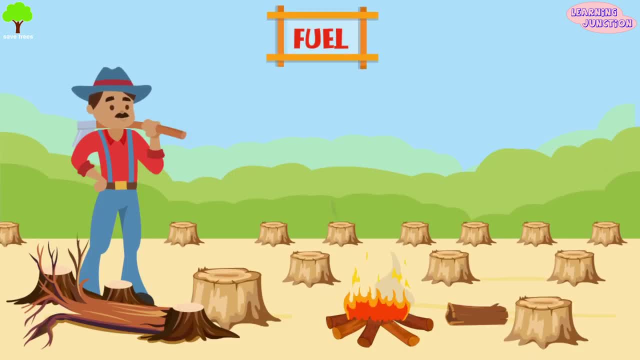 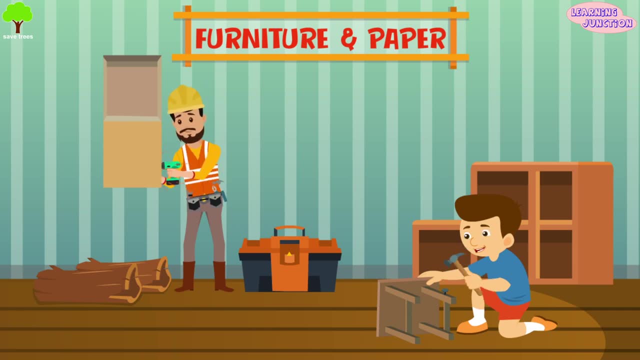 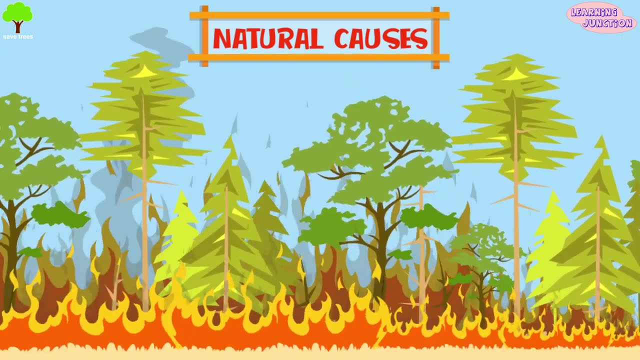 Fuel. Wood from trees is burned And used as fuel for cooking and other activities. Furniture and paper. Trees are cut to obtain wood. Wood from trees is used to make furniture and paper. Natural causes- Deforestation also occurs due to natural causes like forest fires. 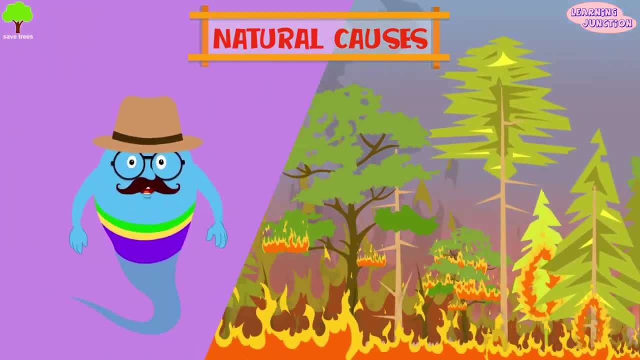 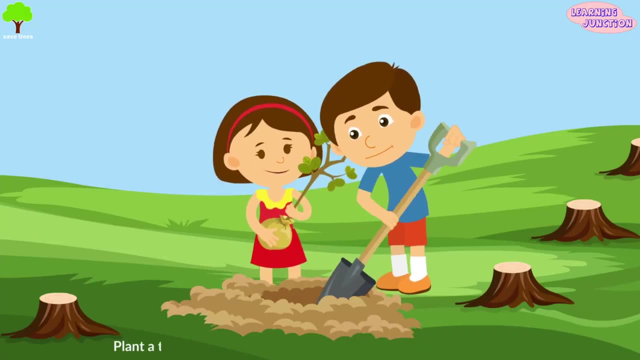 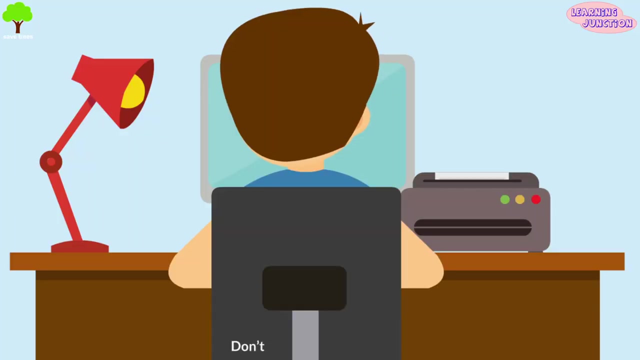 flood, climate change and drought. We should try to stop deforestation. Here are some ways. Very good, buddy, Plant a tree. Growing more trees is the easiest way to help your planet. Don't print unnecessarily. Try to avoid printing any files you're still not sure you really need. 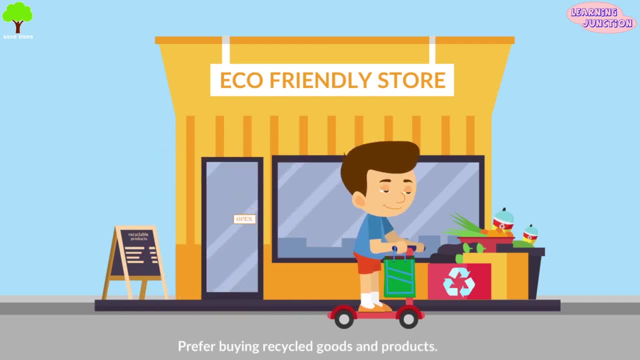 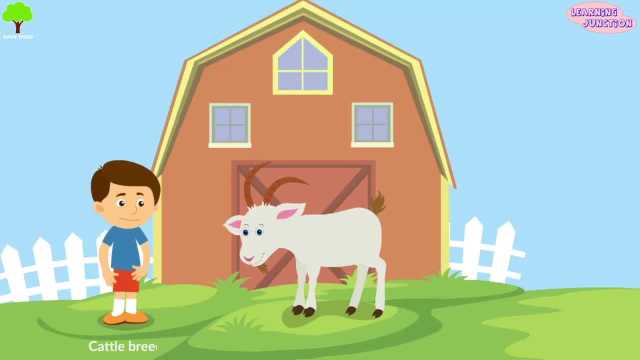 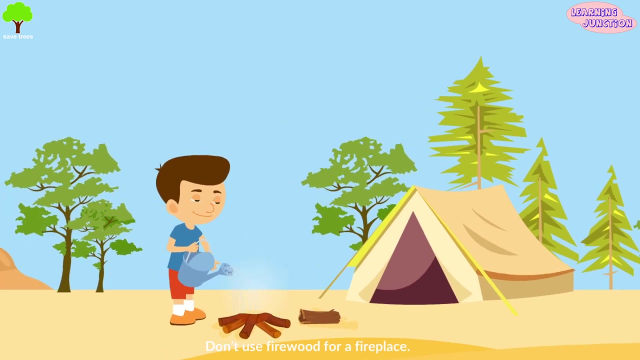 Prefer buying recycled goods and products. A recycling icon on the product means it was made from renewable resources. Cattle breeding requires millions of tons of food of plant of origin each year. Avoid eating meat and save plants easily. Don't use firewood for a fireplace. Make sure your personal comfort and luxury does not harm. 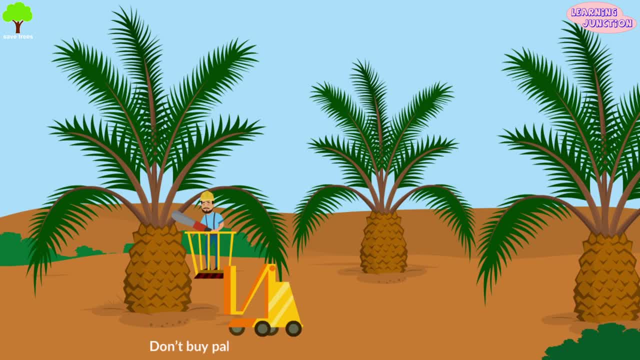 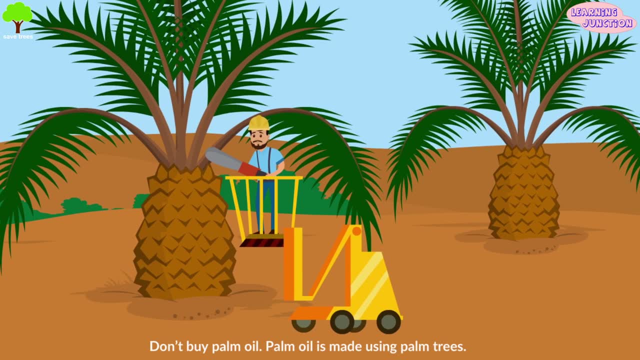 the whole environment. Don't buy palm oil. Palm oil is made using palm trees. Every hour, the area of about 350 football fields of wood is cut off for making this type of oil. A tree is cut off during the season. This is definitely against the law. You shouldn't use it every morning or evening.